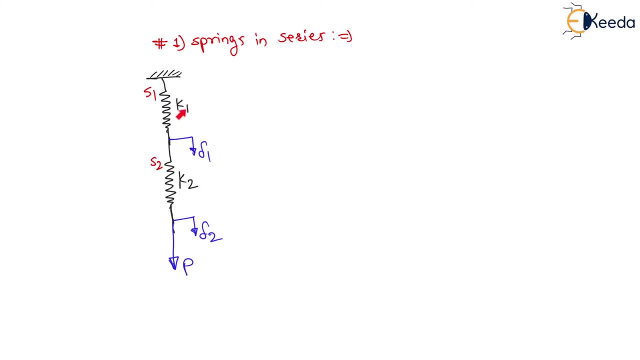 springs And here, in first spring, the spring stiffness K1, which is nothing but force divided by deformation 1.. And in second spring, the spring stiffness K2 will be equal to force divided by deformation 2.. Right Now, instead of using these two springs, if I want to 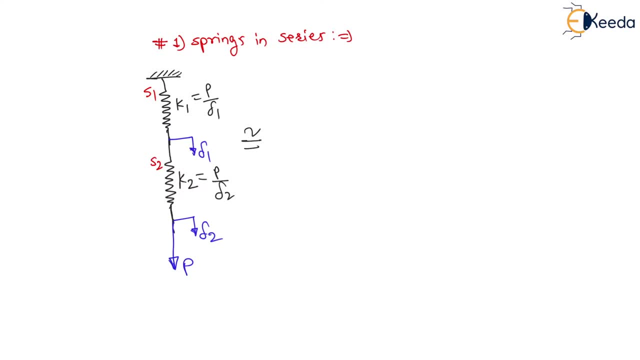 make the spring 1, then I have to make the spring 2.. So I have to make the spring 1 and I have to make the equivalent spring. Here I am making equivalent spring of these two springs in series. Then there will be an equivalent stiffness of this spring. For. 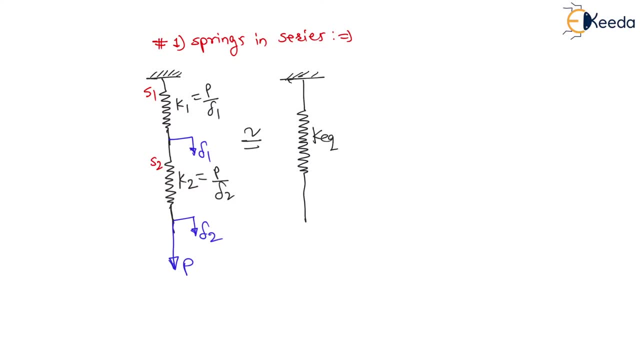 this spring, there will be a K equivalent Right And the force acting on the spring will be the same. The force will be same And this equivalent spring will deform by delta amount Right. This equivalent spring will deform by delta amount. Now, my dear, 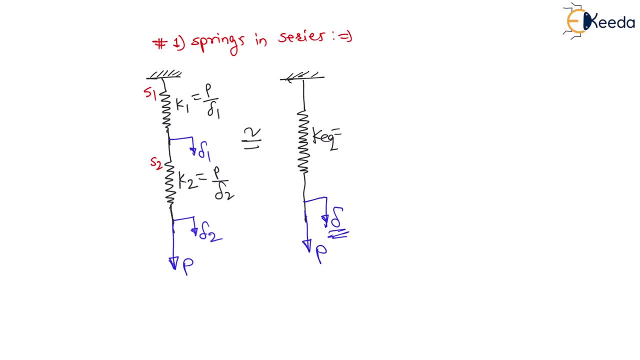 students. definitely this K equivalent will be equal to force divided by deformation 1 and K equal to force divided by deformation 2.. Definitely, Right Now can I say: in all springs, that is, spring 1,, spring 2, as well as equivalent spring, the force is same Right. 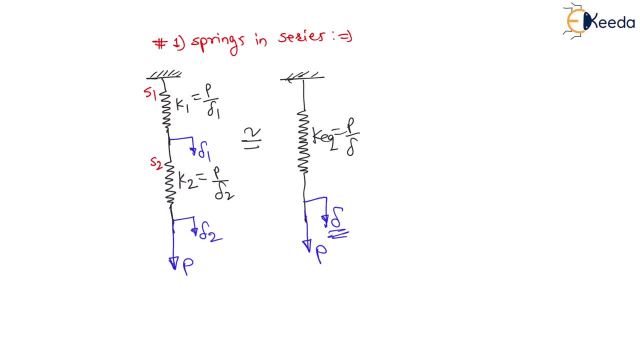 The force is same. Therefore can I say here, as force is same, force is nothing but K delta. Right Force is nothing but K delta, which is same. And here, for equivalent spring, the deformation will be here, deformation of first spring as well as deformation of. 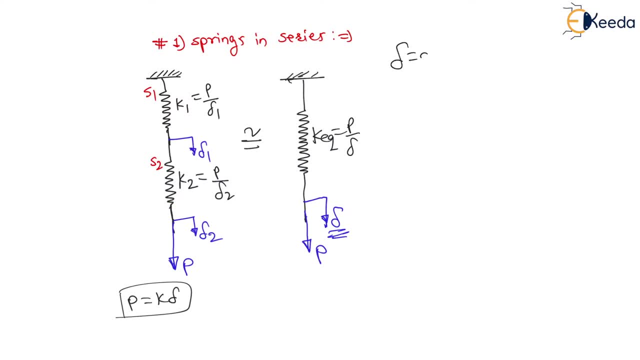 second spring, Right? Therefore, can I say: the deformation will be equal to deformation 1 plus deformation 2.. Definitely we can say: like this, Right? Therefore, my dear students, from this equation we can say: deformation is equal to P divided by K force divided by stiffness. Therefore, 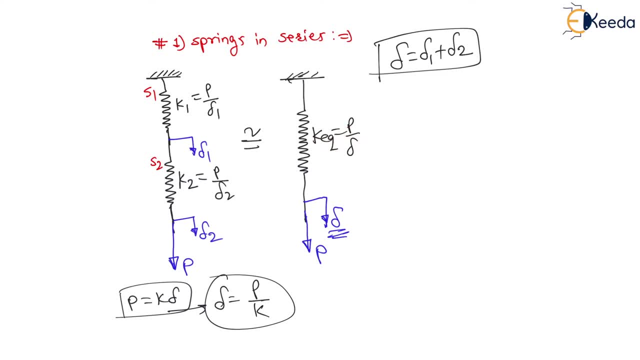 from here for delta it will be K divided by delta is P divided by K, equivalent is equal to delta 1. Delta 1 is nothing but P divided by K 1. P divided by K 1 plus delta 2.. 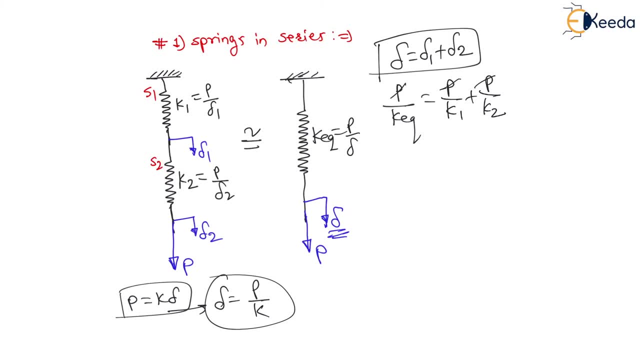 So delta 2 is P divided by K 2. Therefore, from both sides P will get cancelled. Therefore, 1 upon K equivalent is equal to 1 upon K 1 plus 1 upon K 2.. This is how we can find equivalent. 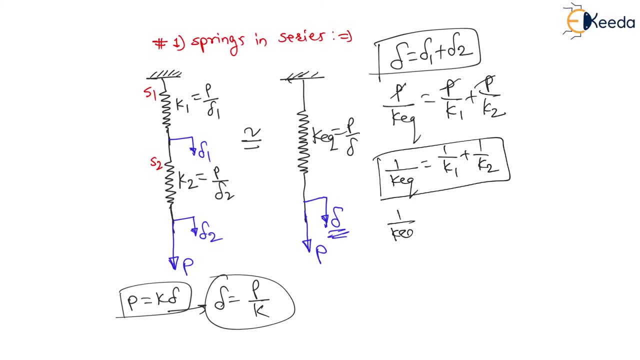 spring stiffness. Again. therefore, 1 upon K equivalent can be written as cross multiply this: K 2 plus K 1 divided by K 1, K 2.. Therefore, K equivalent for two springs in series can be calculated as K 1, K 2 divided by K 1 plus K 2.. This is a shortcut to find equivalent. spring stiffness for K 1, K 2.. So this is how we can find equivalent spring stiffness Again. therefore, 1 upon K equivalent is equal to 1 upon K 1 plus 1 upon K 2 plus 1 upon K 3. 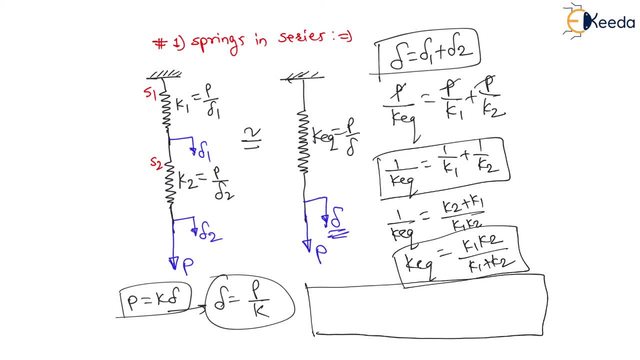 plus so on. Let's say, for the second combination, we have two springs in series. But, my dear students, it is not necessary that there will be only two springs in series. There may be n springs in series. Let's say n springs in series. in series are attached. Therefore. 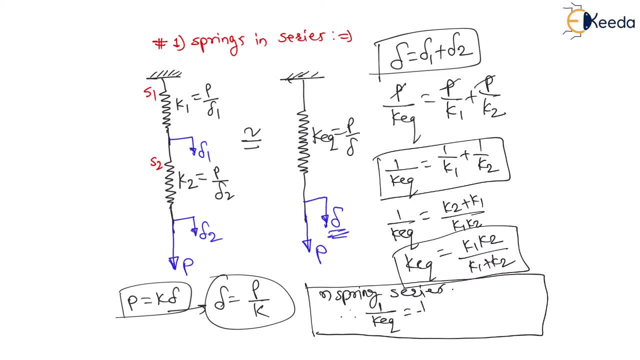 for such cases, 1 upon K equivalent will be equal to 1 upon K 1 plus 1 upon K 2, plus 1 upon K 3, plus so on. whatever may be the number of springs Now, after springs in series, 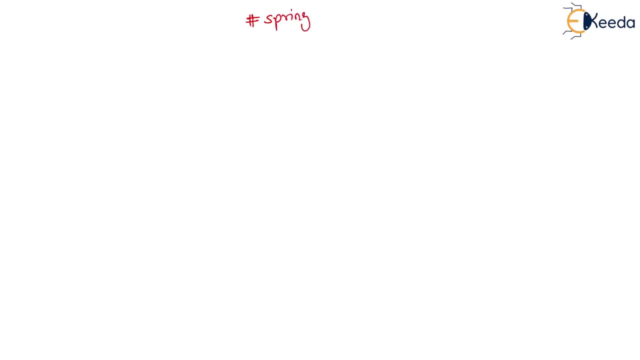 the second combination is springs in parallel, springs in parallel. right, there will be a parallel connection of two springs or three springs, whatever may be the number of springs. now here, let us say the two spring. here my assumption is simple case. let us say: i am assuming there are two springs connected in parallel. let us say this is: 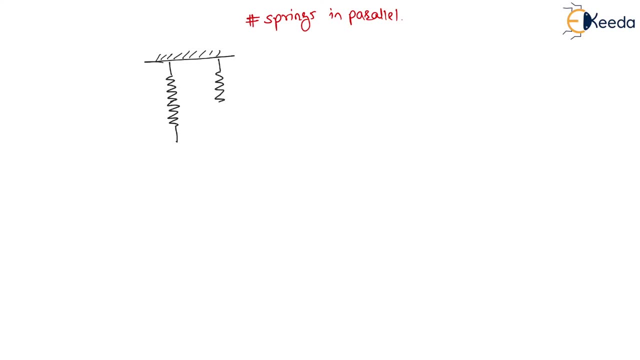 spring, number one, and there is another spring, number two, right. these are the two springs connected in parallel. first spring will be having stiffness k1, second spring will be having stiffness k2 and these two springs are connected in parallel means there will be a common load on. 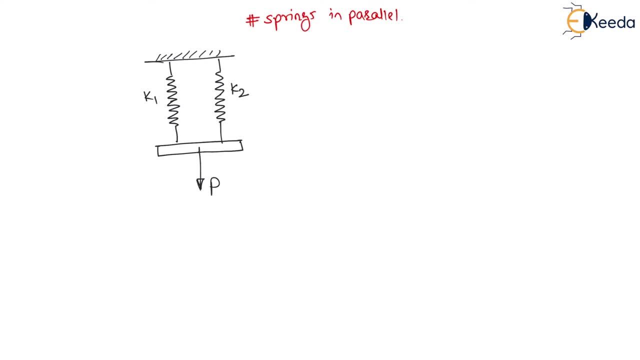 these two springs common load is p, right and, my dear students, parallel connection means the spring will deform by same amount. both springs will deform by same amount means, because of this common load, p, the both spring will deform by same amount. let us say the deformation is here delta. 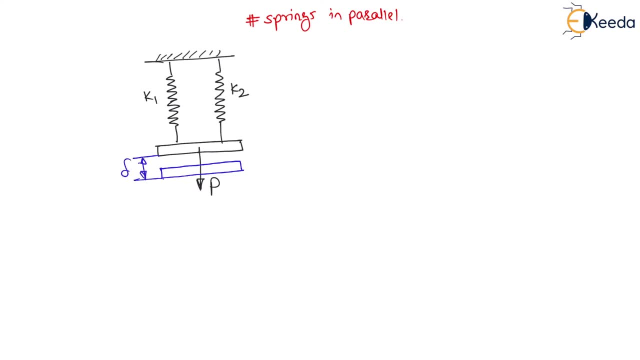 let us say this is the deformation of both springs delta. therefore, here definitely we can say deformation is here delta and this is the deformation of both springs delta. therefore, here definitely we can say deformation is here delta and this is the deformation of both springs. delta of first spring is equal to deformation of second spring right, and these are total force p this. 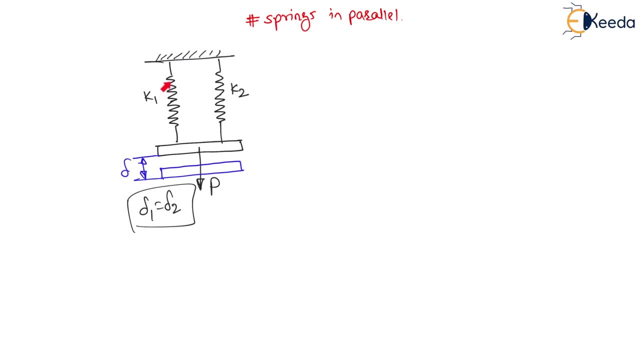 total force p will be shared by spring one as well as spring two. right. therefore, there will be a for resisting this deformation. there will be a reaction in spring one that is force p1 and reaction in spring two that is force p2. therefore, this spring stiffness k1 will be equal to p1 divided by delta.